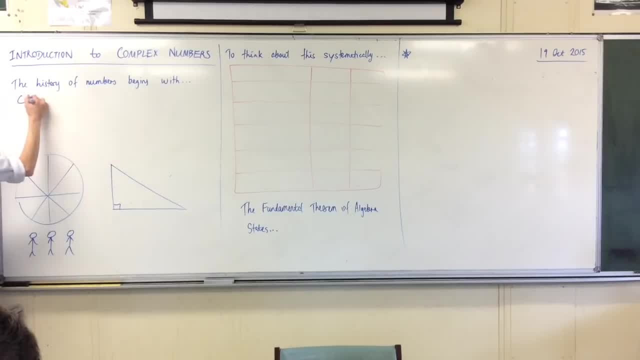 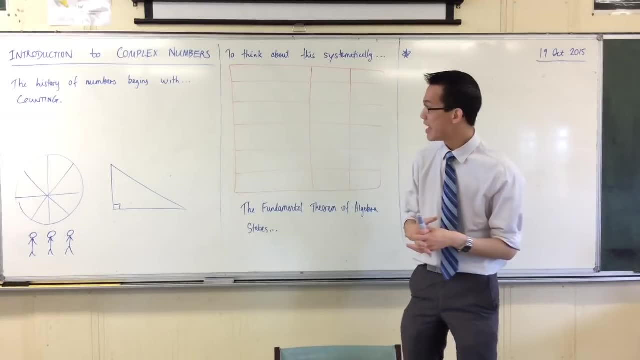 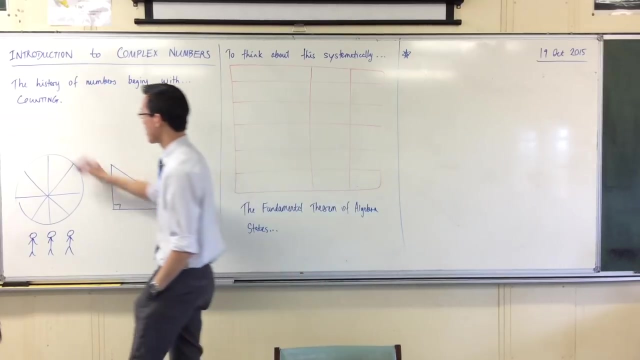 And that context is counting. Now, counting is still something that is evident. The fact that numbers started with counting is still evident in a lot of things that you take for granted. For example, Roman numerals: Right, The first three numbers are written one, two, three. 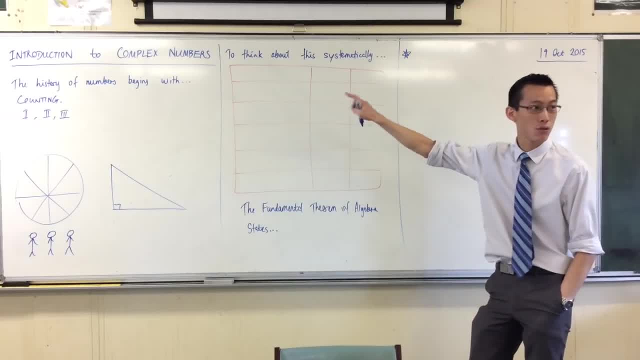 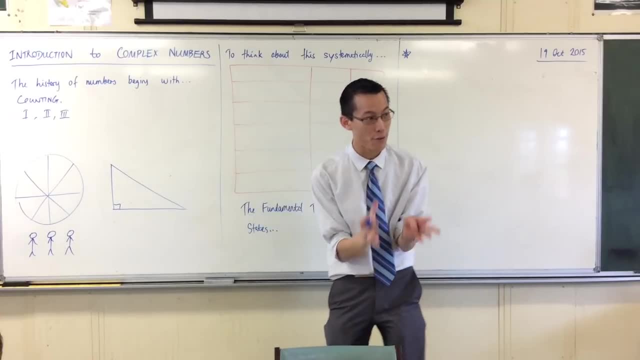 Right. You can see that counting is built into the representation of our numbers. The representation of our numbers- And it's not just the Romans, In fact, more or less every counting system and all the symbols that we use, For example, the Chinese script and the Japanese script, and so on. 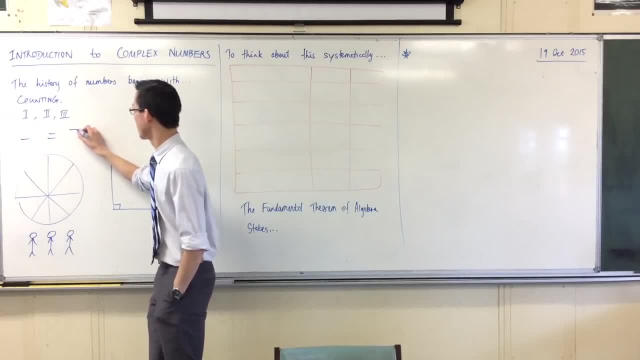 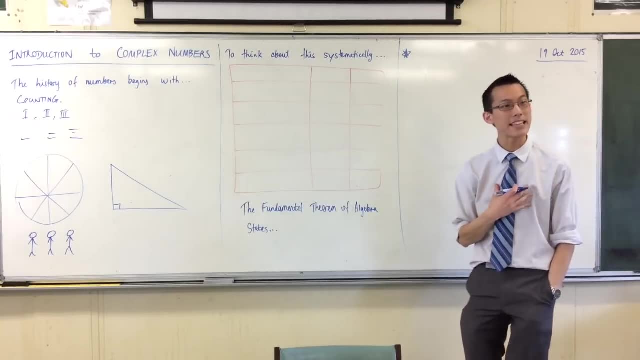 It looks like this: One, two, three. Right, It's got the same pattern of counting, The same pattern of counting built into it And in fact, our numbers. Yes, now four is interesting, Four is- We'll get to four another time. 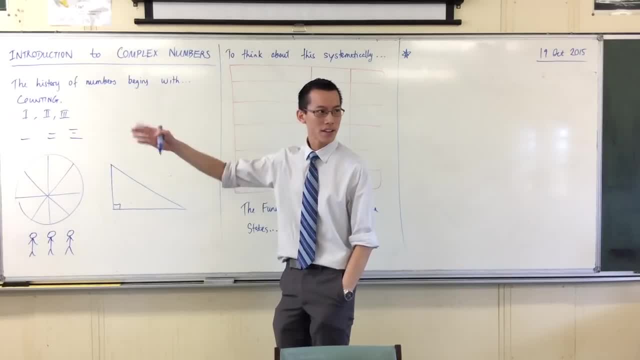 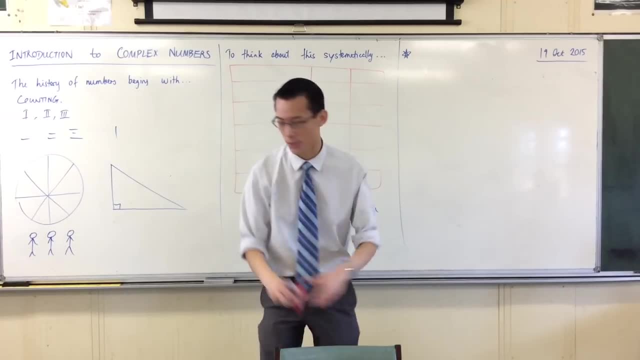 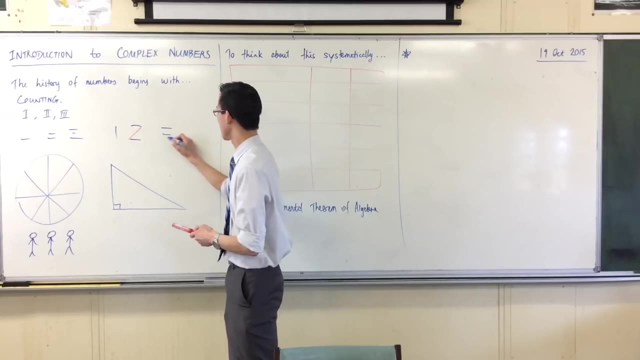 But I just want you to notice. I just want you to notice That one, two and three in this script is not all that different from one. Let me just draw it to make it really obvious: Two And Three In our script, it's not that different. 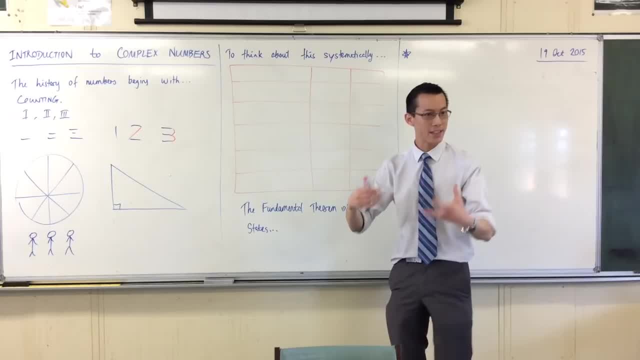 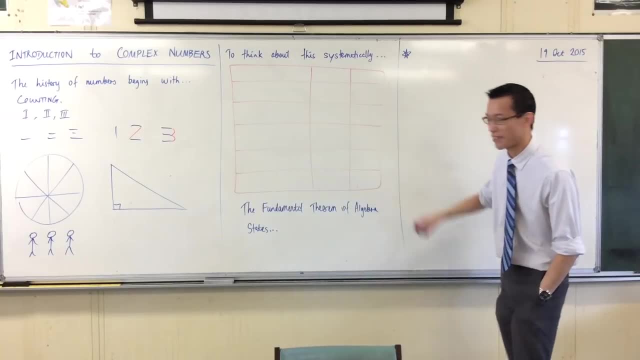 It's just that you've been thinking so long of one and two and three as their own things that you We've sort of not remembered that counting is where they begin. Okay, Question. Okay, We'll move on Now. here's the problem, though. 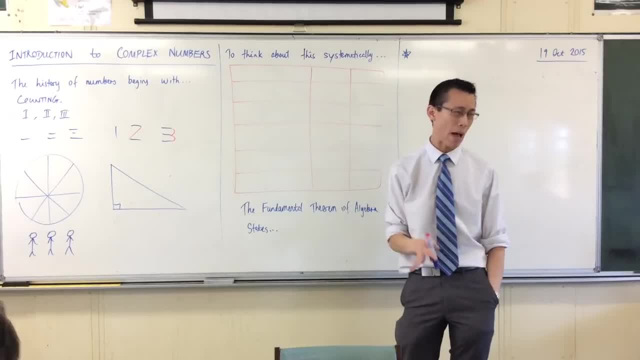 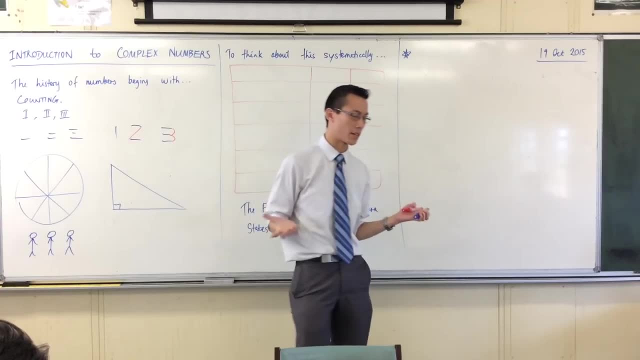 You remember I said that numbers begin with counting, But very rapidly, very rapidly, numbers do not end there. In fact, if you take these numbers, we call them the natural numbers or the counting numbers. it's pretty obvious to see that the natural numbers are not the only kinds of numbers. 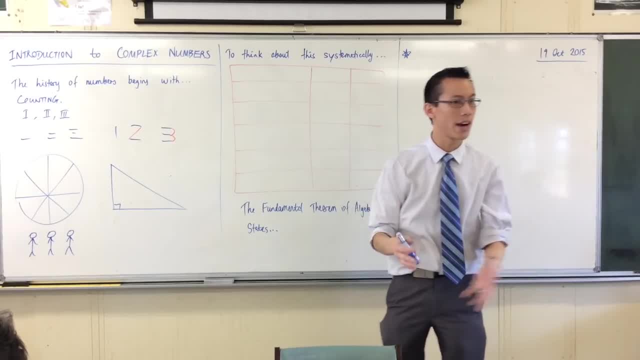 They are, The counting numbers sort of give rise to all these other kinds of numbers, For instance, very simple situations, If you've got like a whole number of objects, a counting number of objects and a whole number of people or groups that you want to separate them out to or share them into. 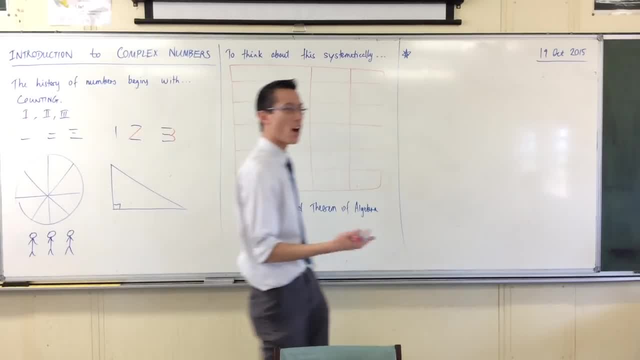 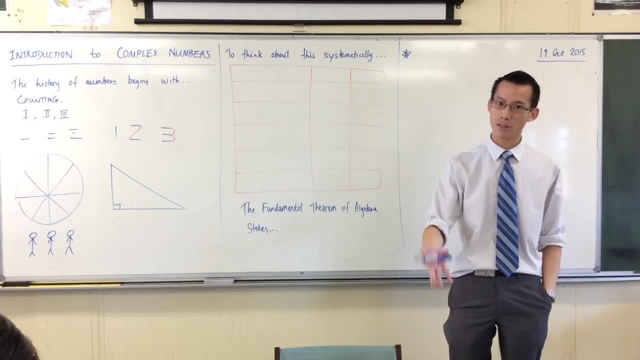 you quickly realise that they don't each get a whole or a counting number of pizza slices right. Eight into three, It doesn't go neatly. It goes into two, It goes into four, It goes into one right, But it doesn't go into three. 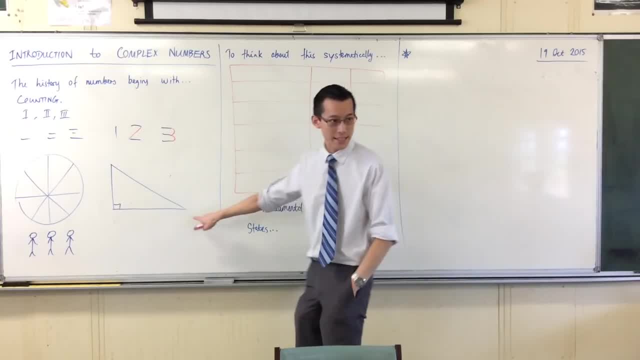 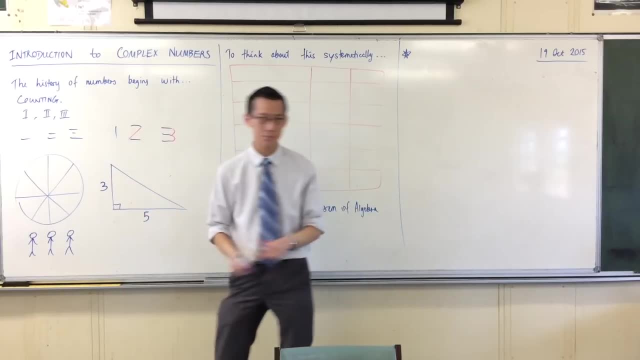 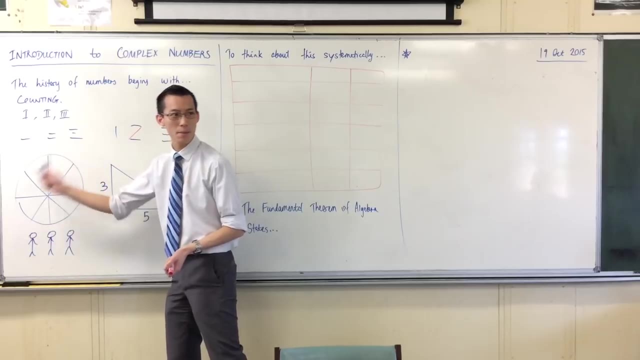 New numbers have to be introduced right In the same way. very quickly the Greeks realised that even if you've got whole number lengths here and here, what you get out here is a different kind of number again. It's not another kind of number like this. 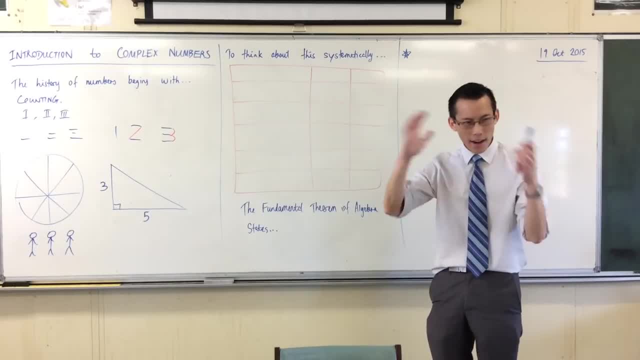 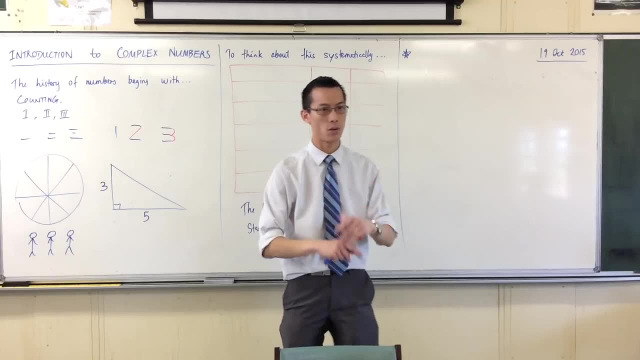 It's not a ratio, It's something different. They argued for a long time as to why. They argued for a long time as to what it was, But they knew it wasn't like these guys. It wasn't a counting number, It wasn't a rational number, and so on. 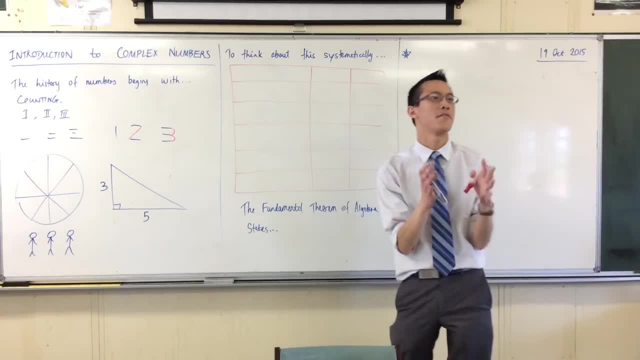 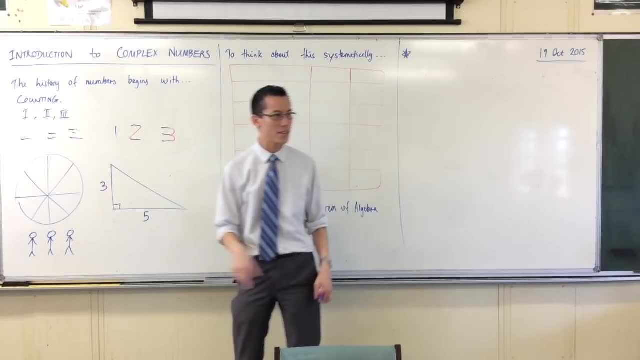 So this whole history of the development of numbers is really about. well, you start here, Everyone starts here, But when you start to combine these in different ways, you start to realise one, two, three, four, they're not enough. 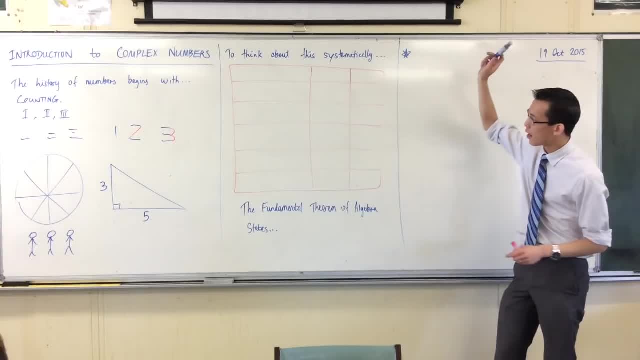 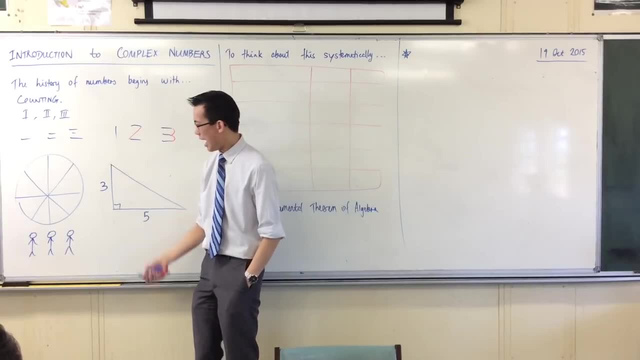 So let's think about this in a systematic way. Draw up this table, if you like. It doesn't have to be big. So what we're doing here, like starting with counting and then talking about division- That's what this is, isn't it? 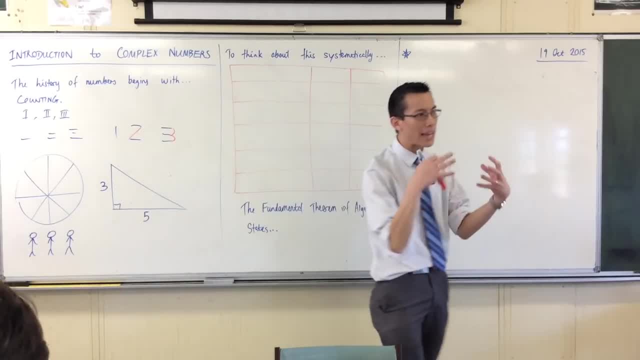 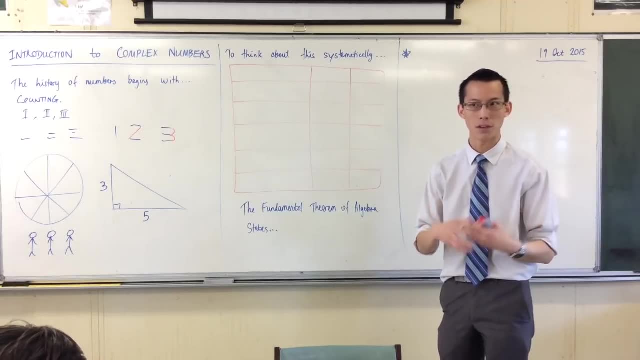 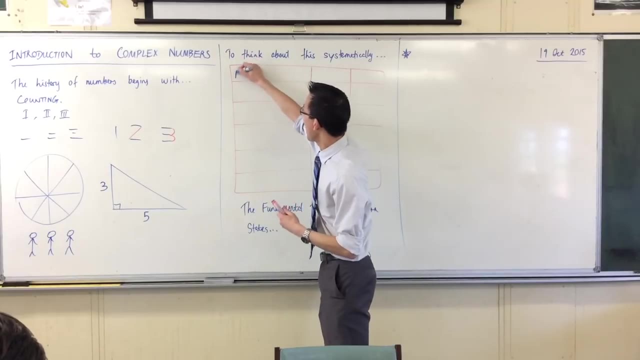 Or talking about these lengths and so on. What binds all these ideas together is that we manipulate them through algebra. We manipulate them through the laws and rules of algebra and the operations. So what we're going to put together here is a series of algebraic equations. 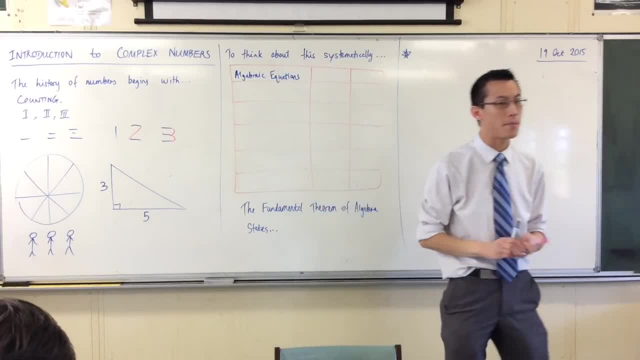 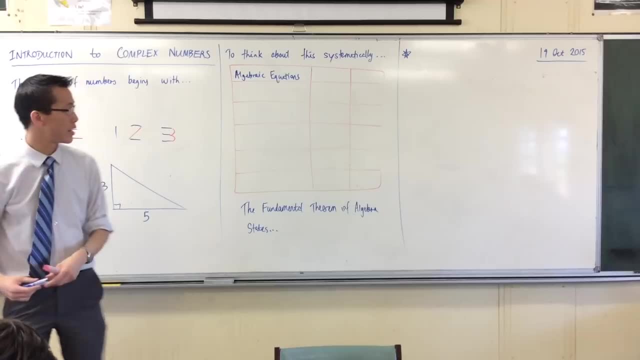 We're going to use these familiar counting numbers. Those are our building blocks And you'll see if we combine them in ways- and you already know about these ways- mostly If we combine them with plus, minus, times, divide and indices. 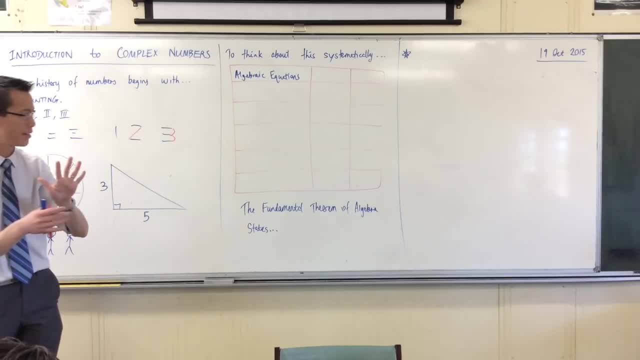 Exponentiation, which is very, very similar- Not entirely identical, but very similar- to the idea of repeated multiplication. If you just take these five algebraic operations right, Then you will see all of these different kinds of numbers. They fall out. 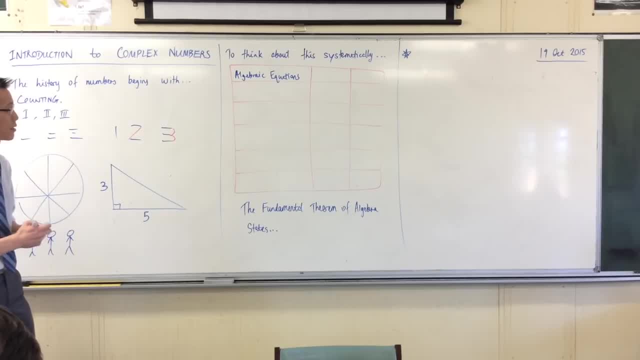 I want to give you some language and some notation to describe these. So, for instance, if we think of a simple equation like x, take away 5, equals 0. There's an equation for you. It has an answer. There's a solution to this right. 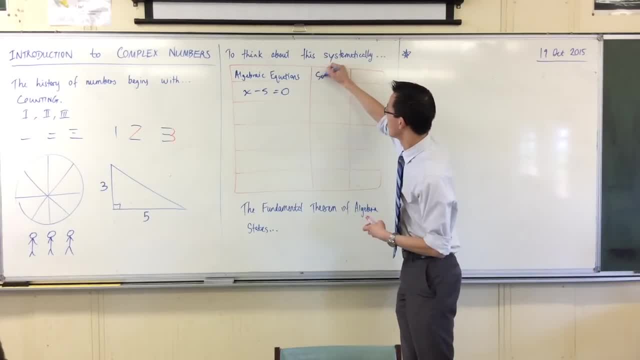 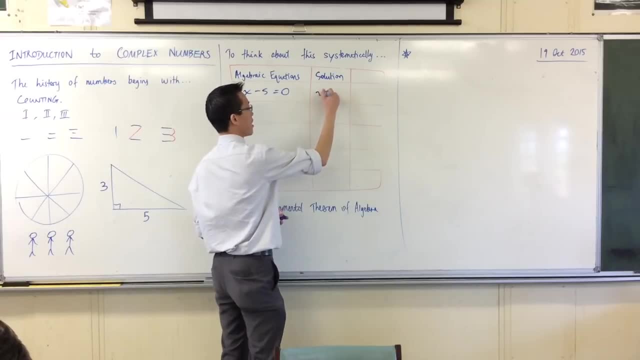 Or a root, if you like. The solution, of course, to x minus 5 equals 0 is x equals 5.. It's x equals 5.. Very good, So this is our simple example. This is still back in this region of counting numbers, right. 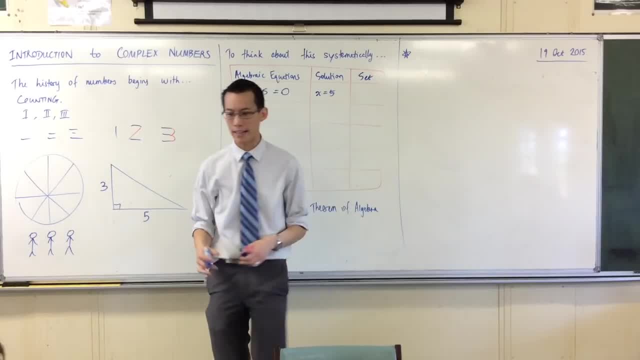 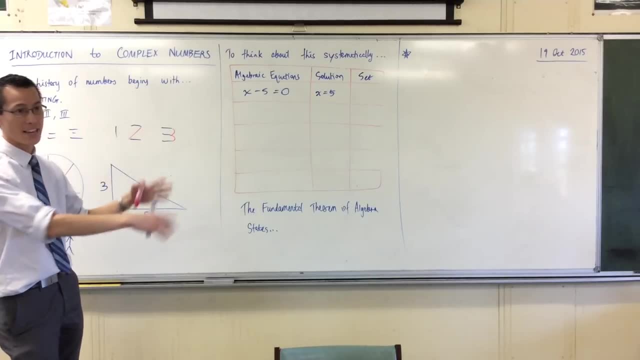 But I want to get some more fine language and notation on this, Because, as we've talked about before, language is power. Once you know how to describe something which you have language to describe it, you can understand it, manipulate it, interpret it and so on. 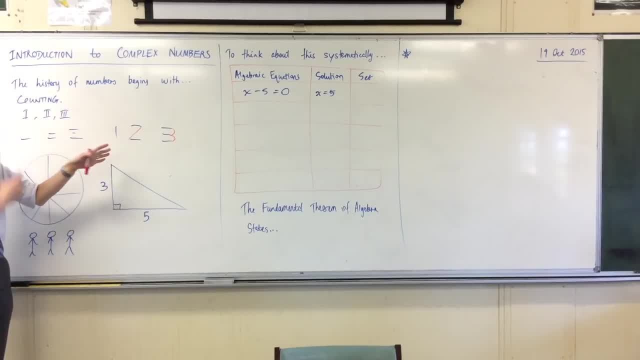 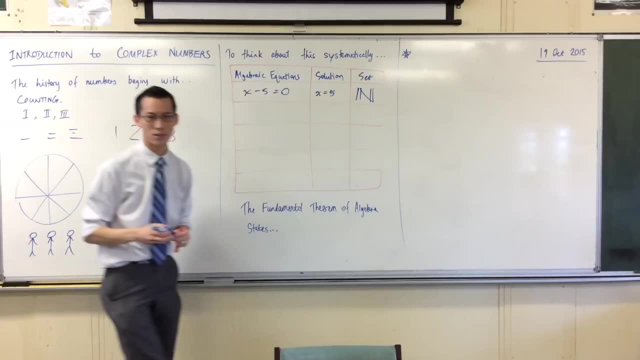 So these counting numbers, our technical name for them are the natural numbers, The natural numbers, And we have a symbol for it. I have showed it to you before. I think It's an N with extra lines on it: N for natural. 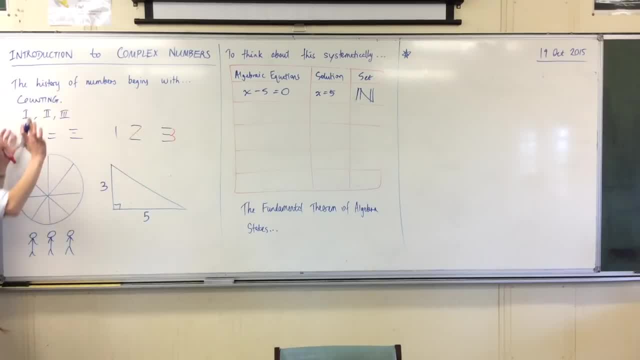 Alright, that's pretty simple. That's it. That's in our counting number world. But it's pretty easy to get out of the counting number world, For instance, if I give you an equation like this, which is just as simple: 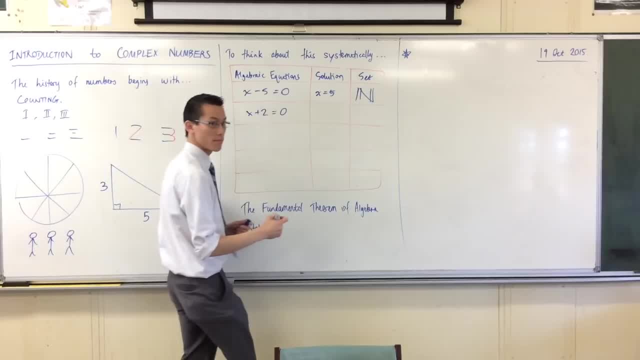 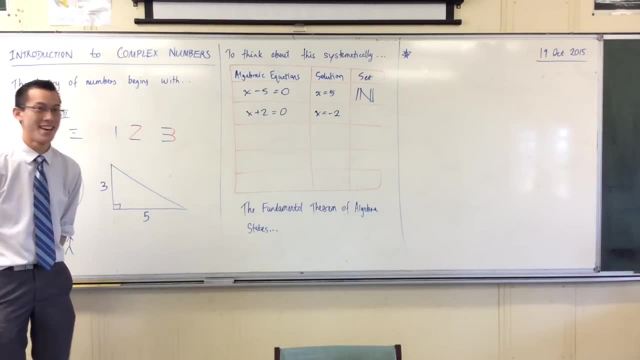 Just as simple. What's the solution? x equals negative 2, right, So we are pretty quickly like. I haven't even gone past addition and subtraction, right? I'm out of the counting number world already. right Now. negative 2 is not a counting number. 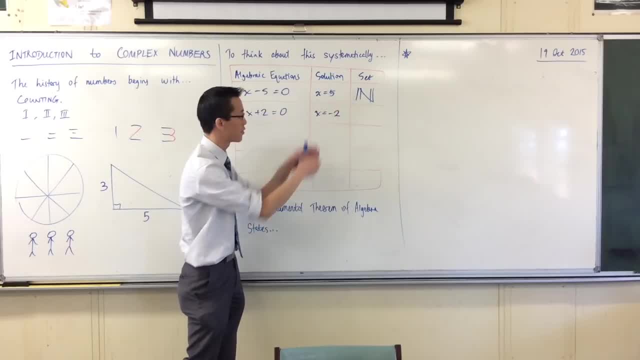 It's not a natural number in the technical sense of the word. We have another name for this. Starts with an I. We call it integers. okay, Now, for reasons that will become clear in a second, even though the name of it is integers. 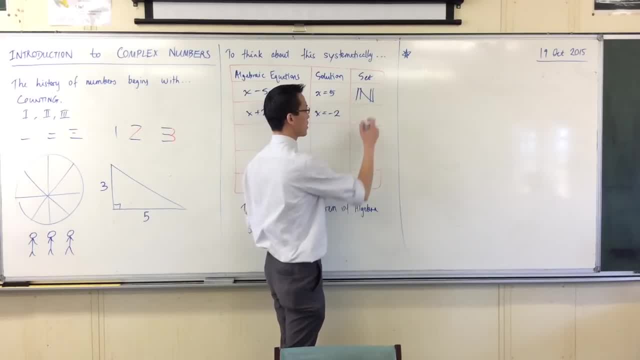 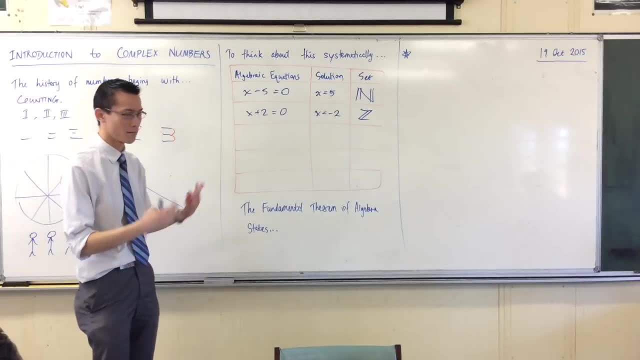 we don't use an I here. We use the character z, which we get from the Germans. It's an abbreviation of the German word zahl, which means, ironically, counting. but anyway, These are the integers. That's the name, That's the symbol that you will see attached to integers. okay, 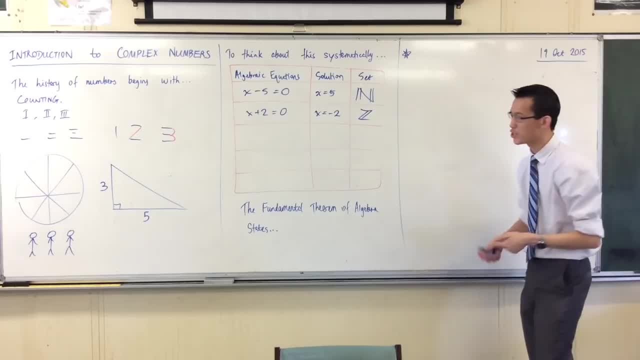 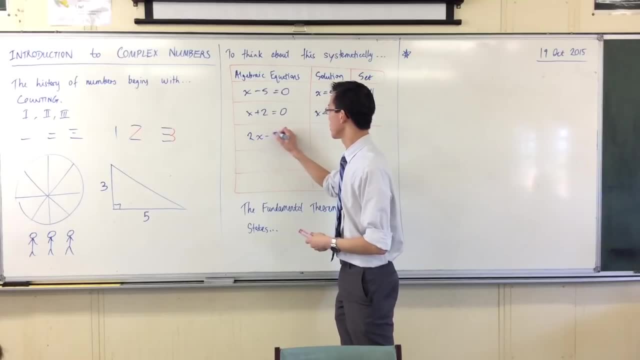 All right Now. we went past the natural numbers, We went past integers. If we stay with using the counting numbers to construct this thing, for instance- again another simple equation, something like this: What is the solution to this algebraic equation? 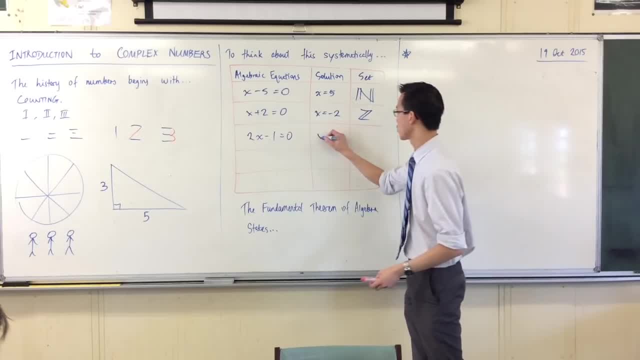 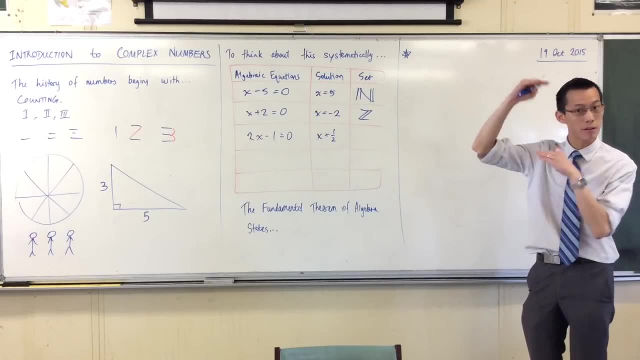 x equals a half, right x equals a half. Now, this is still in familiar territory for us. This is a rational number. okay, It's a ratio between 1 and 2.. Our symbol for this, again for reasons that will become clear in a second, we do not use. 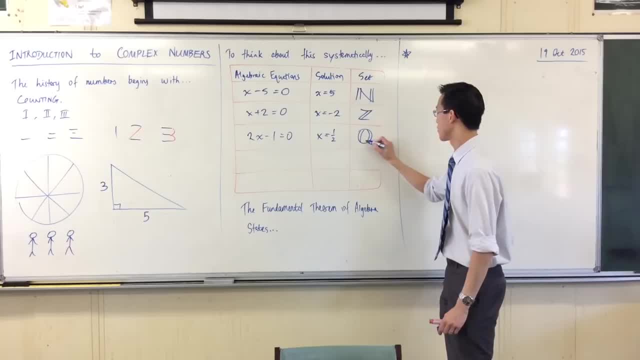 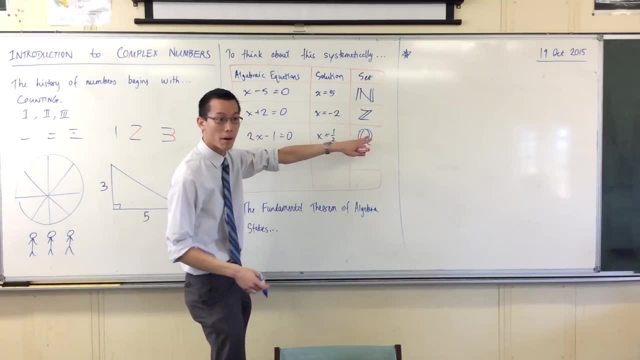 R for rational, We use a Q, which stands for not rational. but what word? Quotient? Yeah, thank you. Quotient, right, This is a division number, because that's kind of where it begins, where we get these rational. 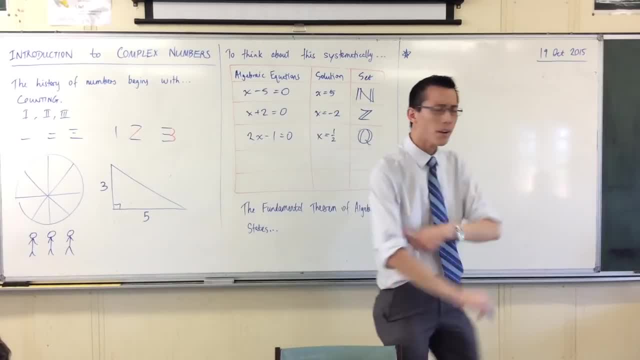 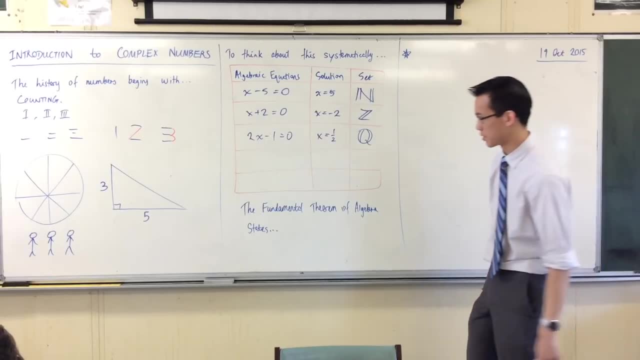 numbers from Q for quotient. Okay, Now there's one last category of numbers that we have been dealing with over the last many number of years. okay, And I can quickly come up with a solution, an equation that will give me this something. 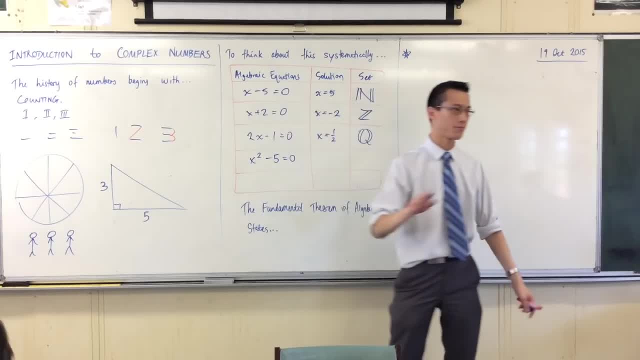 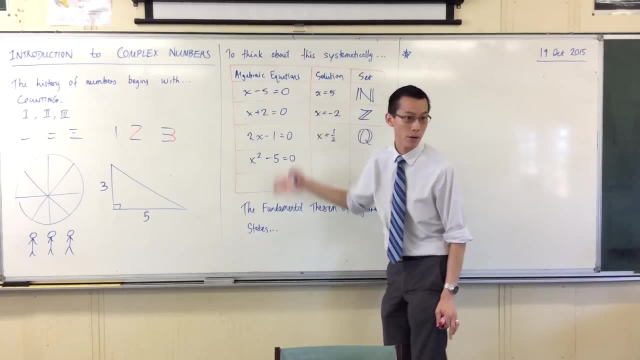 like say, let's do this, So I've gone to exponentiation here, so I've got an index. but, importantly, all of my numbers that I've used to build my equations, they're all counting numbers, right, Like these are still the building blocks, but you combine them in simple ways and you 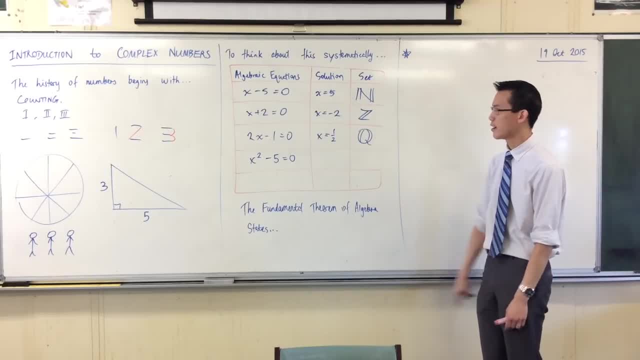 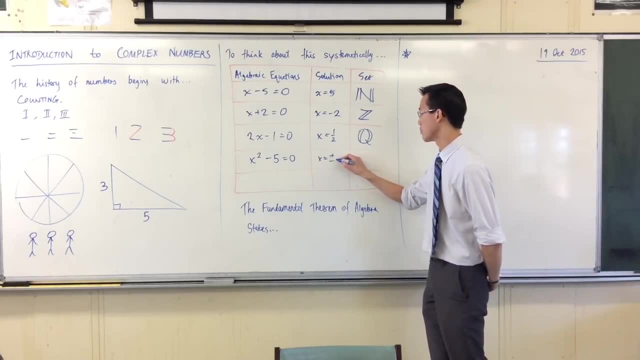 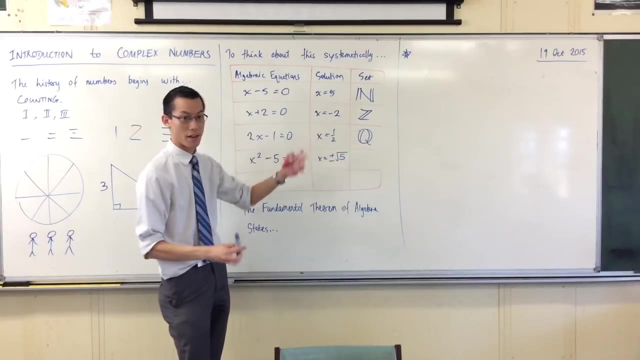 get weirdo different numbers over here. What is the solution, or rather, what are the solutions to this equation? Okay, so x equals plus 4 minus the square root of 5,. okay, Now square roots where the number that's underneath the square root isn't a square. 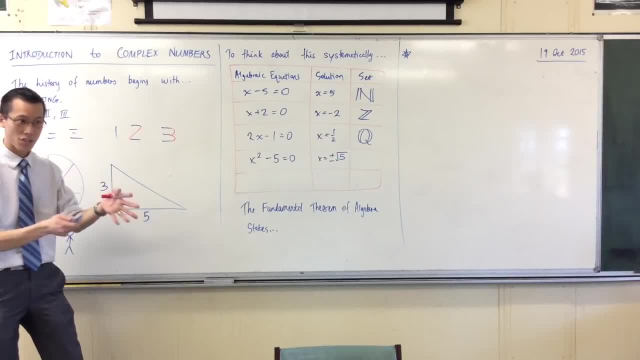 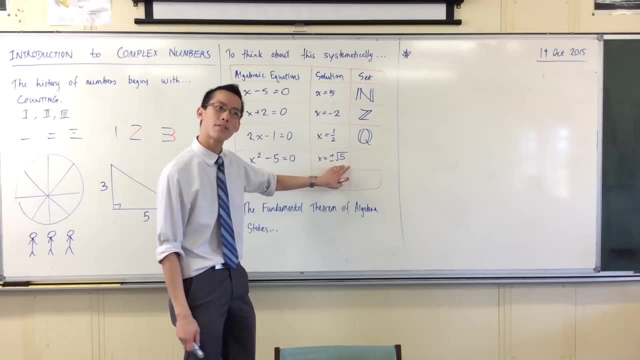 number. these are not rational numbers, You can't write them. There's no fraction that this is equal to right, At least no fraction that's just built with counting numbers. So therefore this is a different kind of number. 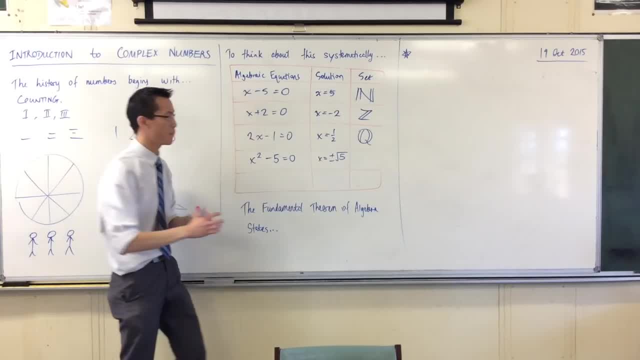 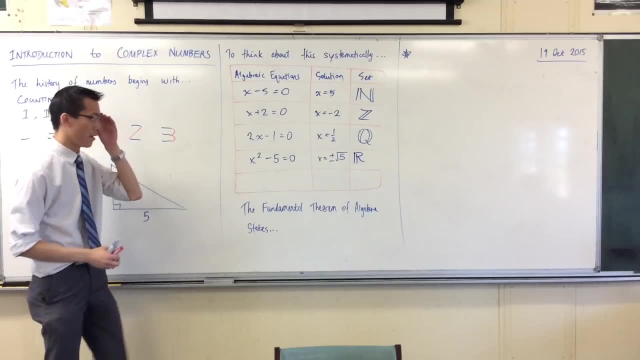 It's irrational, right, But more widely speaking, it belongs to this class of numbers: The real numbers, The real numbers. Okay, So we've been talking about this for a long time. We talked about quadratics that have real solutions or don't have real solutions, right. 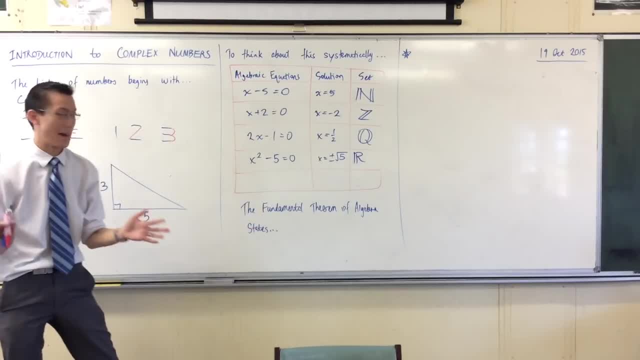 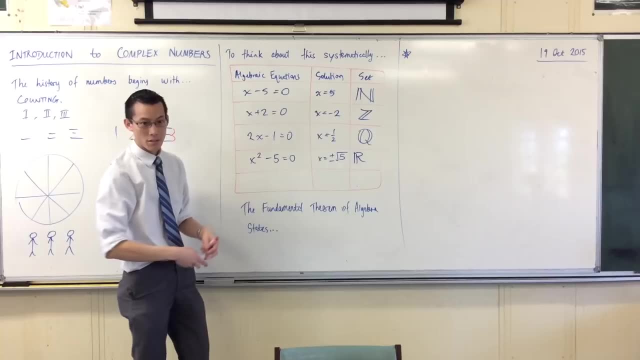 Now, this has taken us a long way, where you can do a lot of maths with real numbers- okay, But it doesn't quite take us all the way. Think about algebraic equations, right, And these simple tools that we've been using to build solutions, right.